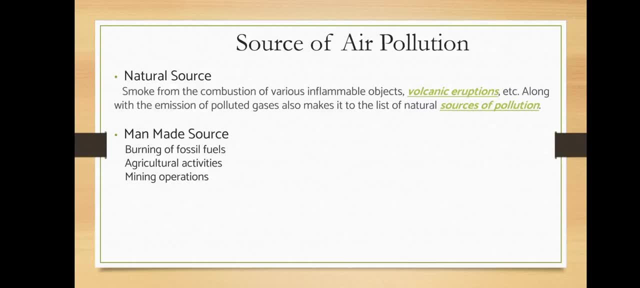 Third: ozone deflection And the next is source of air pollution. Source of air pollution are two types: natural source and man-made source. Natural source: smoke from the combustion of various inflammable objects, volcanic eruption, etc. Along with the emission of polluted gas, also make. it is the list of natural source of pollution. 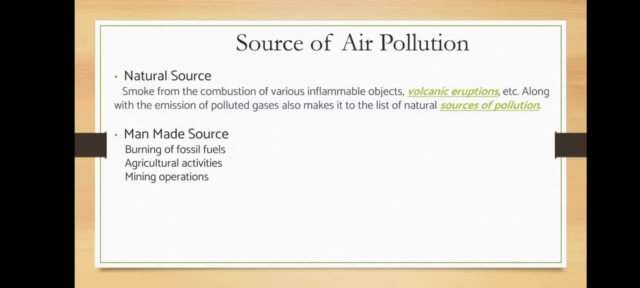 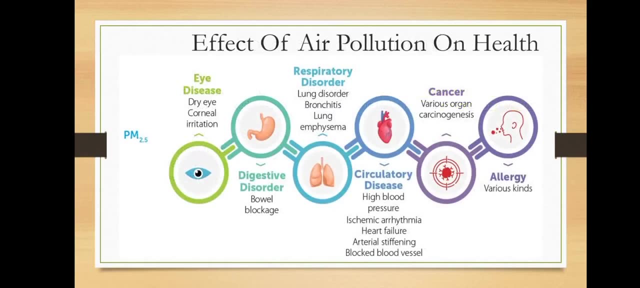 And second is man-made source: burning of fossil fuel, agricultural activities, mining operations. And the next is effect of air pollution on health. First, particulate matter 2.5, eye disease, digestive disorder, respiratory disorder, circulatory disorder, cancer, algae. 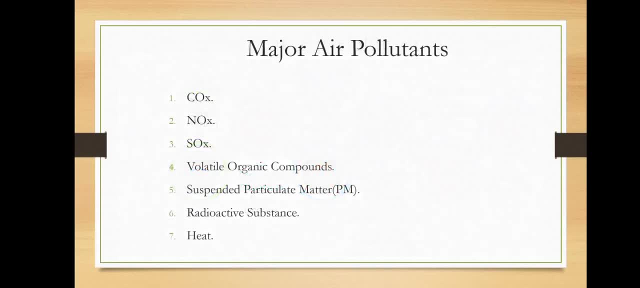 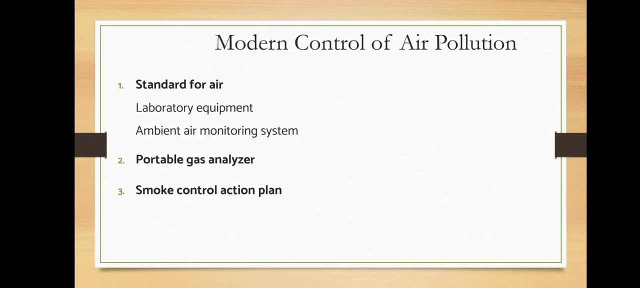 And the next is major air pollutants: carbon oxides, and second in nitrogen oxides, third is sulfur oxides and for volatile organic compound and fifth suspended particulate matter and six is radioactive substance and seventh heat. and the next is modern control of air pollution, basically modern air control. pollution are three types standard of 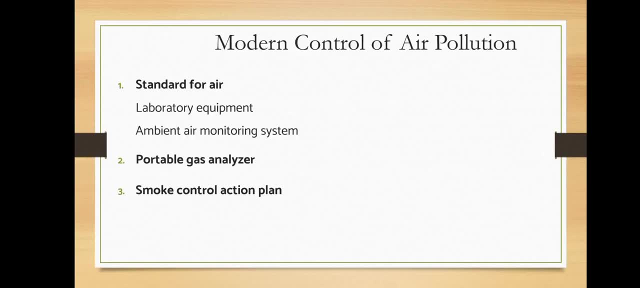 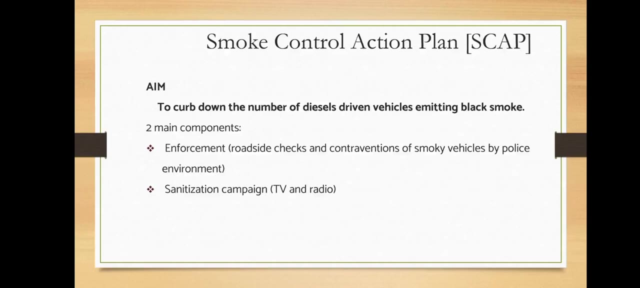 air. standard of air are two types: laboratory equipment, eminent air monitoring system. and second is portable gas analyzer. and third is smoke control action plan. and the next is smoke control action plan- short form escape aim to curve down the number of diesel drive-in vehicles emitting black smoke. are two main components: first, enforcement. 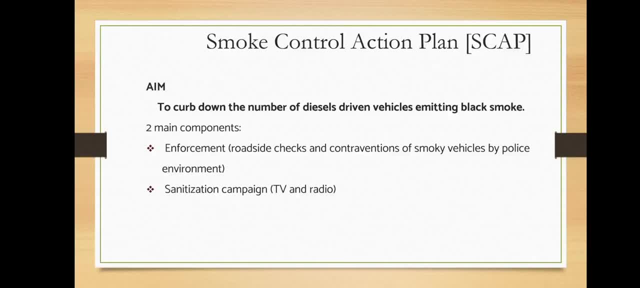 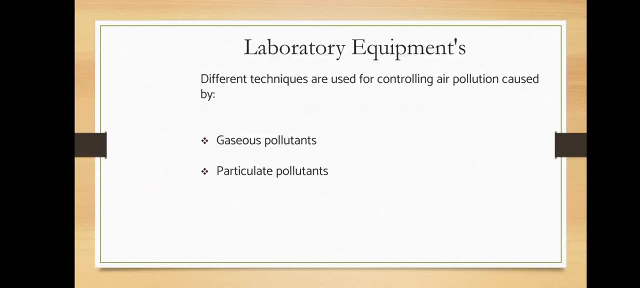 roadside check and convention of smoking vehicle by police involved or meant the second in St Jason, champion TV and radio. and the next is laboratory equipment. different technique are used for controlling air pollution caused by gaseous pollutants, but plate pollutants. and the next is method of 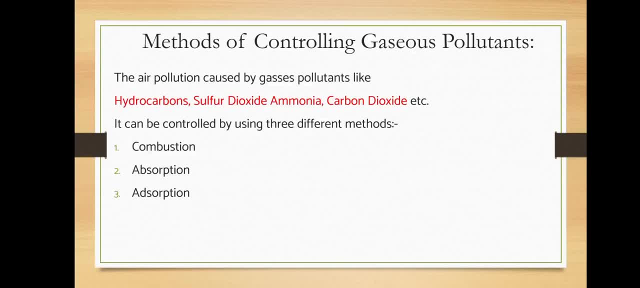 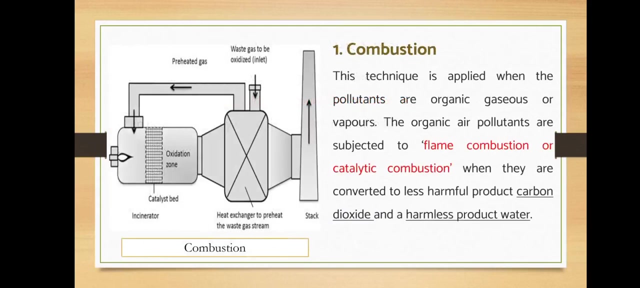 controlling gaseous pollutants: the air pollutant caused by gaseous pollutant like hydrocarbon, sulfur dioxide, ammonia, carbon dioxide, extra by the organic gases, it can be controlled. for clean air pollution it can be controlled by using three different methods: forced combat, combustion, absorption. adsorption- first combustion: the technique is 힘들ified. 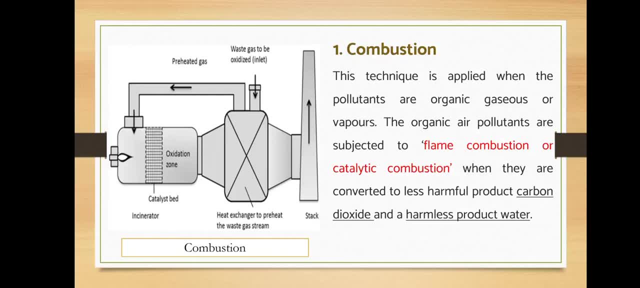 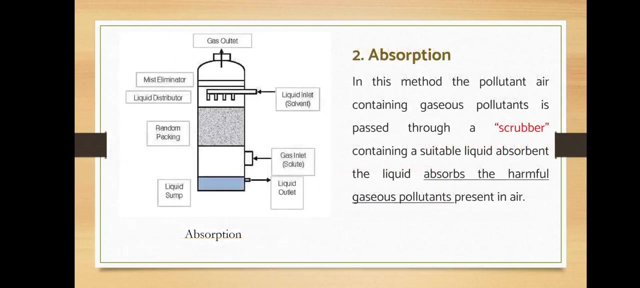 when the pollutants are organic, gaseous or peppers, though organic air pollution, are subjected to flame combustion, but catalytic combustion when they are converted to less harmful produce, product carbon dioxide and harmless product water. now see the figure, our process here and second absorption. in this method, the pollutant air containing gaseous pollutant is processed out. 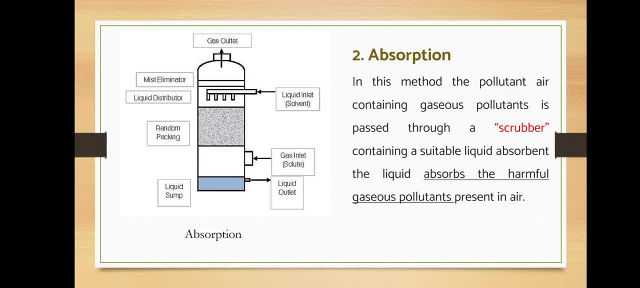 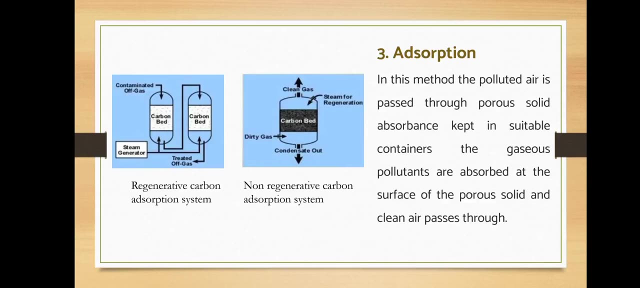 scrubber containing is a to have a liquid have to absorb and the liquid absorbed the harmful gases pollutant present in air and toddy's add drops, son, in this matter. the pollutant air is process out for a solid absorbs. kept in suitable container, the gaseous pollutants are absorbed at the surface. 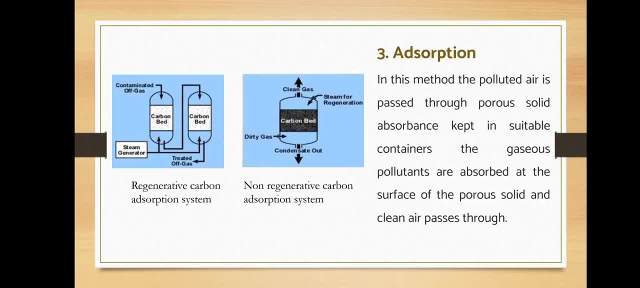 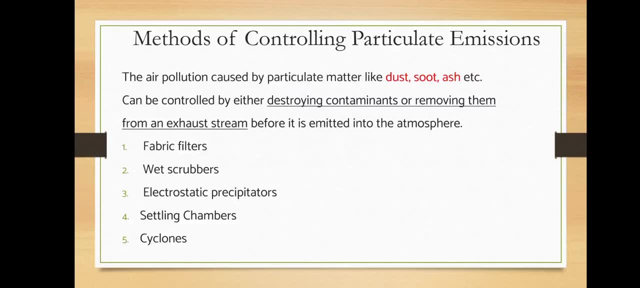 of products. solid and clean air: fastest route- now see the figure. and next is: now see the figure. and next is: now see the figure. and next is: absorb the harmful gaseous pollutant present in air. and third is adsorption: Methods of controlling particulate emission, The air pollution caused by particulate matter. 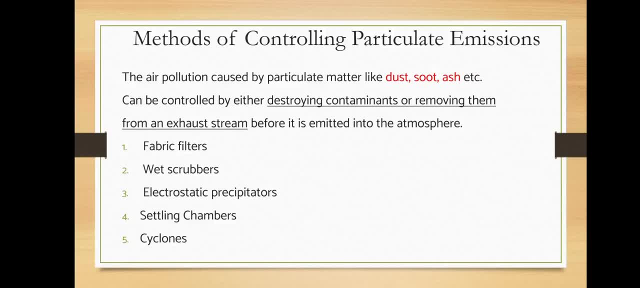 like dust soot ash, can be controlled by either destroying contaminants or removing them from exhaust stream before it is emitted into the entire atmosphere. Here are five types of methods of controlling particulate emission: First, Fibric filters. second, wet scrubber. third, electrostatic precipitator. fourth, settling. 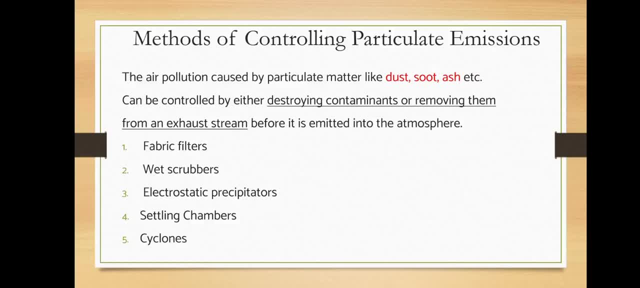 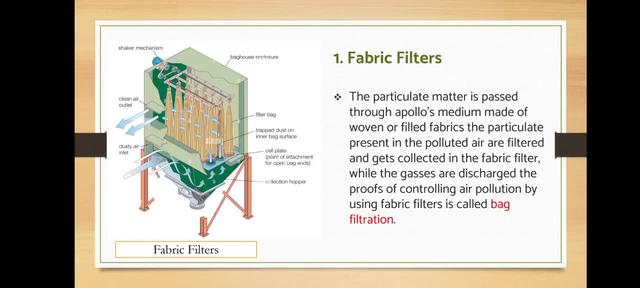 chamber. fifth cyclones Now see first type Fibric filters. The particulate matter is passed through a porous medium made of oven or fillet fabrics. Particulate present in the pollutant air are filtered And gets collected in the fibric filter. 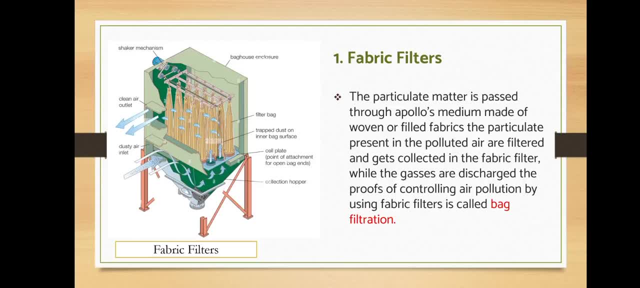 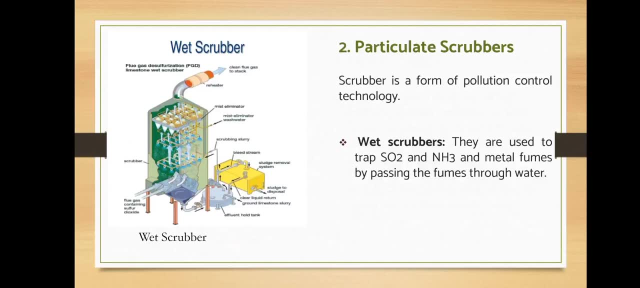 While the gases are discarded. the proof of controlling air pollution by using fibric filters is called back filter. And second is particulate scrubber. Scrubber is from pollution control technology, Wet scrubber. They are used to trap SO2 and NH3 and metal flume by passing the fume throughout water. 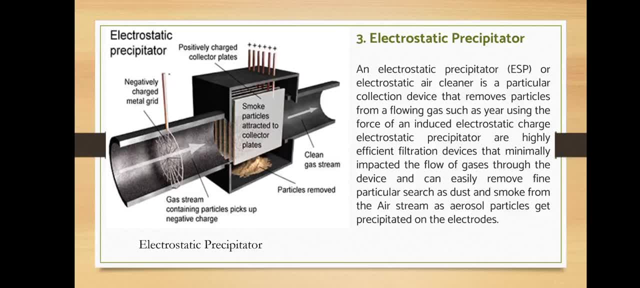 And third is particulate scrubber. They are used to trap SO2 and NH3 and metal flume by passing the fume throughout water. And fourth is electrostatic precipitator. An electrostatic precipitator, or electrostatic air cleaner, is a particulate collection device. 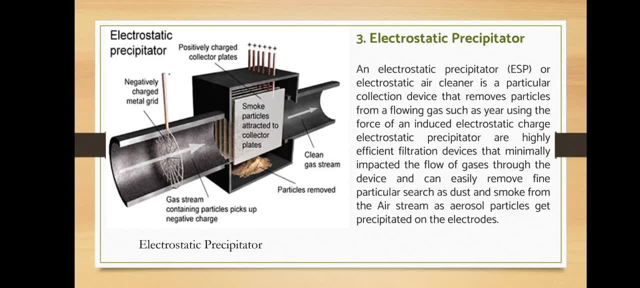 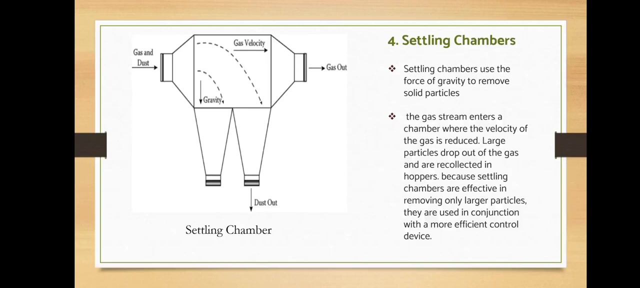 that removes particulate from following gases, such as air, using the force of an induced electrostatic charge. Electrostatic precipitator is a highly efficient filtration device that minimally impacts the gases throughout the device and can easily remove fine particles. And fourth is settling chamber. 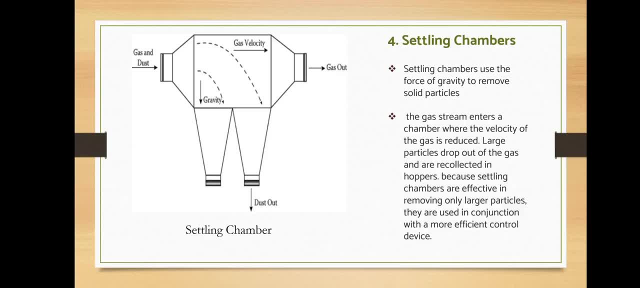 Settling chamber uses the force of gravity to remove solid particles. The gases stream into a chamber where the velocity of gases is reduced. Large particles drop out the gases and are re-collected in hoppers. And fourth is settling chamber. Settling chamber uses the force of gravity to remove solid particles. 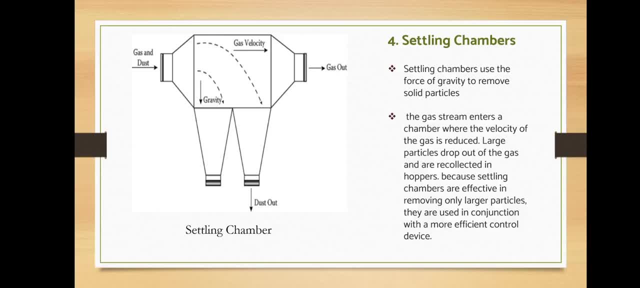 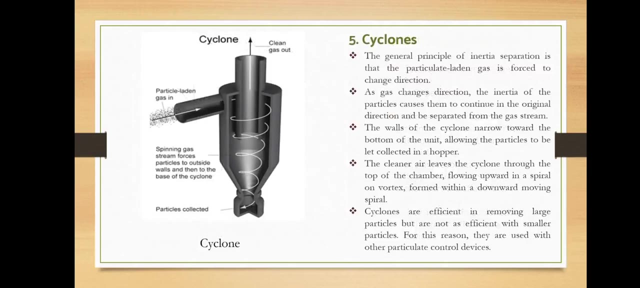 Settling chamber is effective in removing only larger particles. They are used in conjunction with a more efficient control device. Now see the figure in process: settling chamber. And fifth is cyclones. The general principle of inertia separation is that particulate laden gas is forced to. 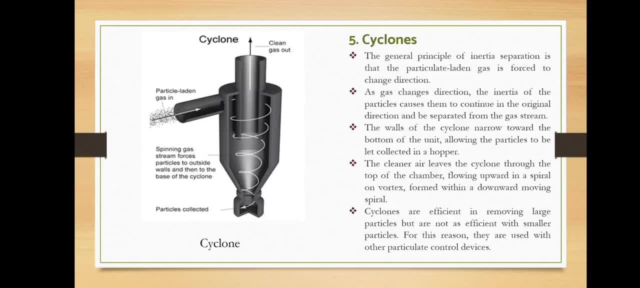 change direction. A gas changes direction. the inertia of the particulate causes them to continue in the original direction. This is separated from the gas stream. The wall of cyclone narrow toward the bottom unit, allowing the particle to be let collected in hopper. 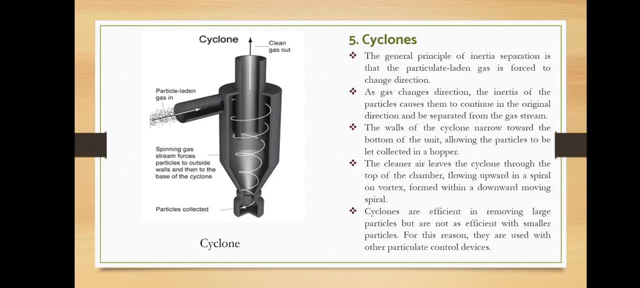 The cleaner air lifts the cyclone throughout the top of chamber flowing upward, a spiral or vortex formed within down-moving spiral Cyclones are efficient in removing large particles, but are not efficient with smaller particles. For this reason, they are used with other particulate or other devices. 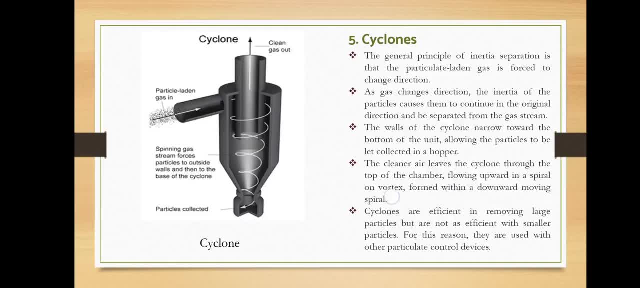 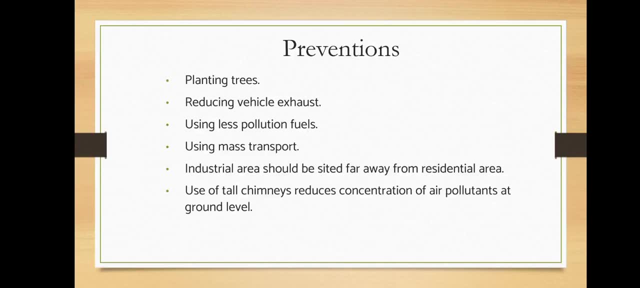 And this is the end of this video. Thank you for watching. And the next is prevention. Planting trees reduce vehicle exhaust using less pollutant fuels. using mass transport, Industrials should be sited away from residential area. Use of tall cinemas reduce concentration of air pollutants at ground level. 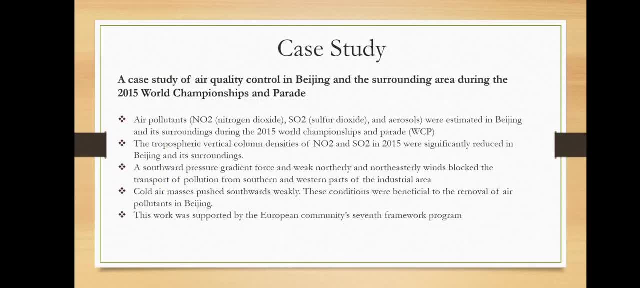 And the next is cache study: A cache study of air quality control In Beijing and the surrounding area during the 2015 World Championship and PRAD. air pollutants- nitrogen dioxide, sulfur dioxide as well- as were estimated in Beijing and its surrounding during the 2015 World Championship and PRAD. the tropospheric vertical column. 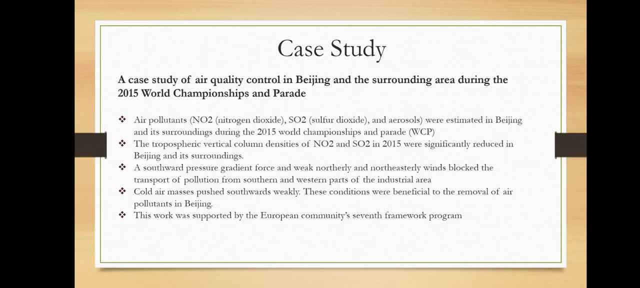 densities of nitrogen dioxide and sulfur dioxide in 2015.. This is the end of this video. Thank you for watching. In the next video, you will learn how batch fall has generated fission installings aggressively reduced in Beijing and its surroundings. 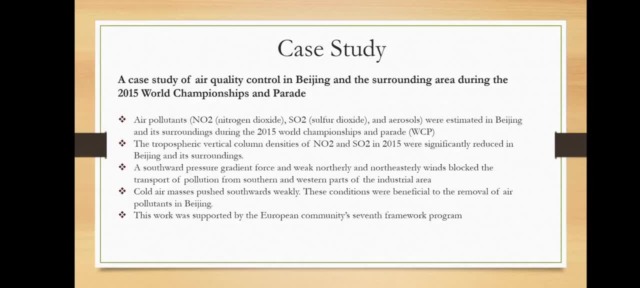 A southward pressure, gradient force, a weak north and a North-East wind block the transport of pollution from the southern and western parts of industrial area. Cold air masses wash out south-ward weakly. This condition is beneficial to the removal of air pollutants in Beijing. 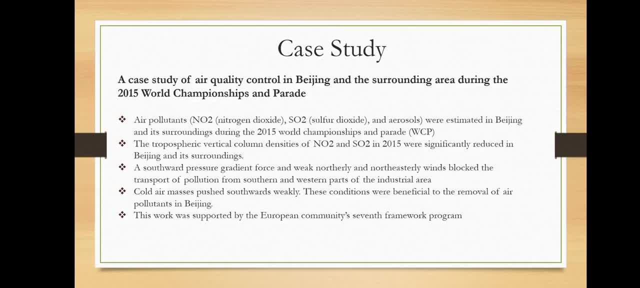 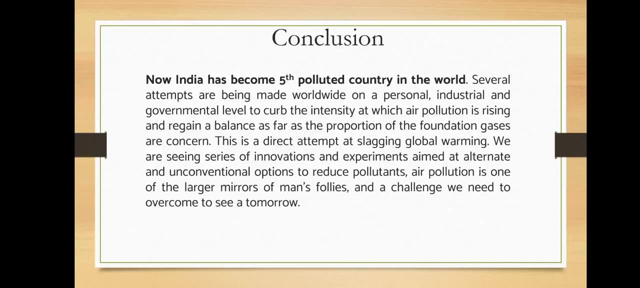 This work was supported by European Community 7th Framework Program. And the next is Conclusion. Conclusion on Modern Air Pollution Control Technologies. Now India has become 5th polluted country in the world. Several attempts are being made worldwide, on personal, industry and governmental level. 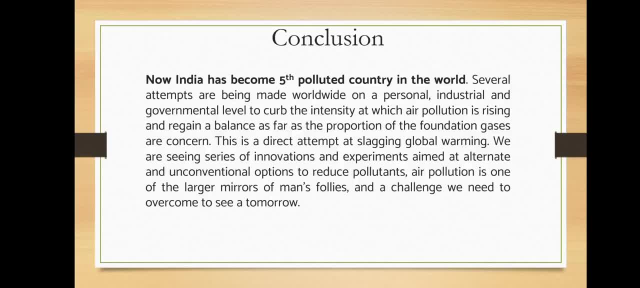 to curb the intensity at which air pollution is rising and region balance. As for the professional of foundation gases are concurrent. This is direct attempt at slashing global warming. We are seeing the series of innovation and experiment having to alternate and unconventional, optional reduced pollutants.